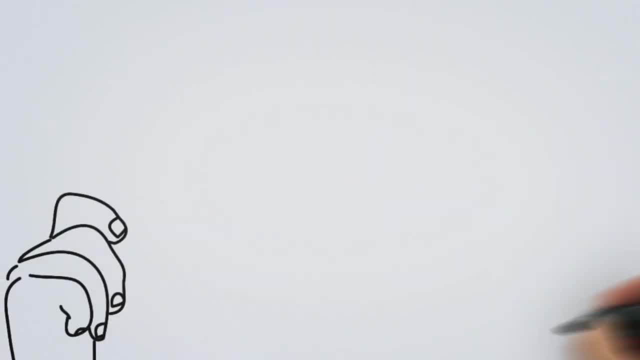 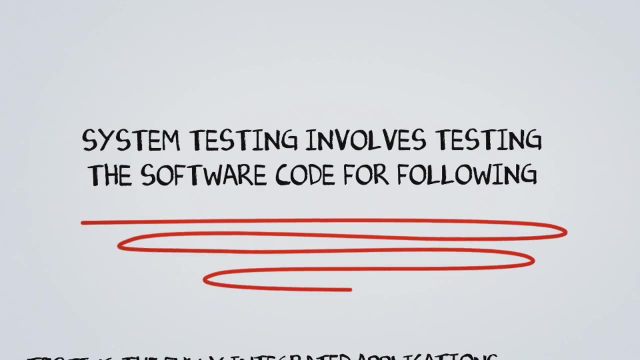 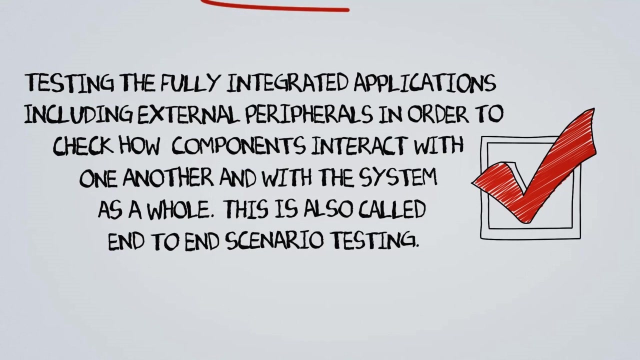 What do you verify in system testing? System testing involves testing the software code for the following: Testing the fully integrated applications, including external peripherals, in order to check how components interact with one another and with the system as a whole. This is also called end-to-end scenario testing. 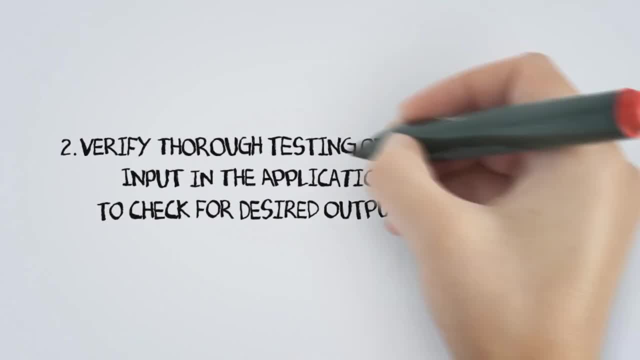 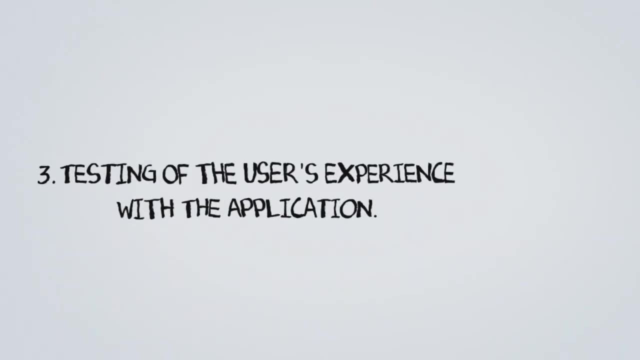 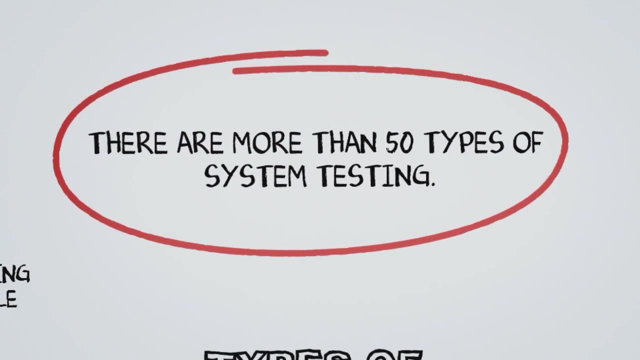 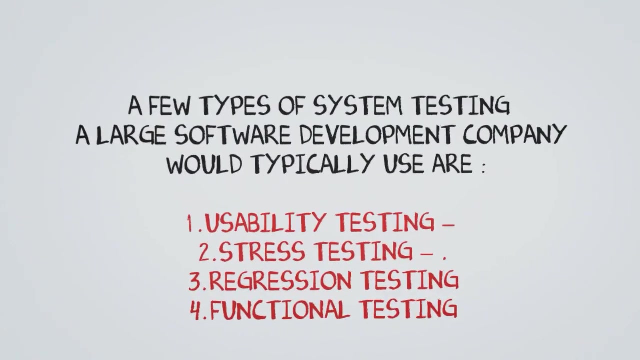 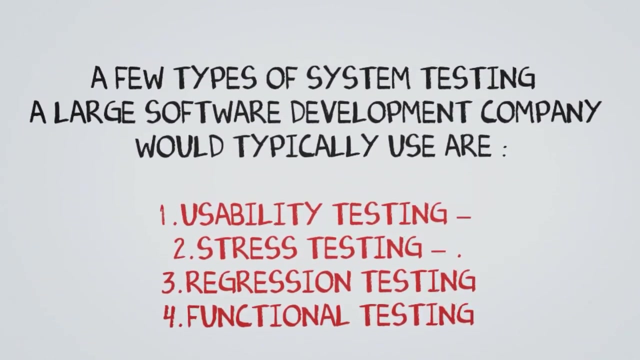 Verify through testing of every input in the application Test, the application to check for desired outputs And testing of the user's experience with the application. Types of system testing. There are more than 50 types of system testing. A few types of system testing a large software development company would typically use are usability testing, stress testing, regression testing and functional testing. 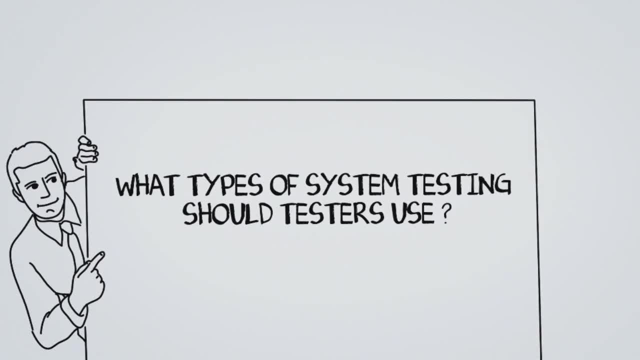 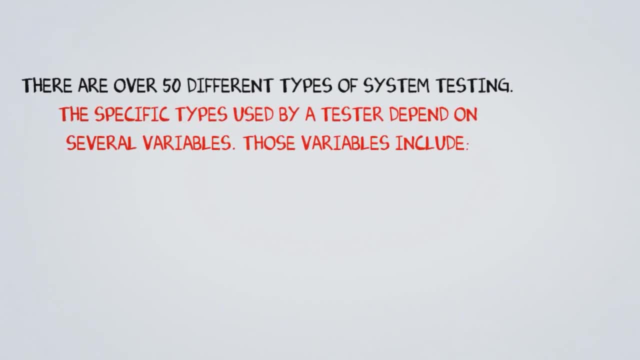 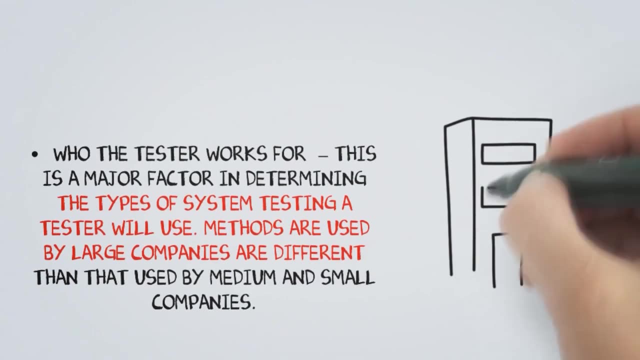 What types of system testing should testers use? There are over 50 different types of system testing. The specific types used by a tester depend on several variables. Those variables include Who the tester works for. This is a major factor in determining the types of system testing a tester will use. 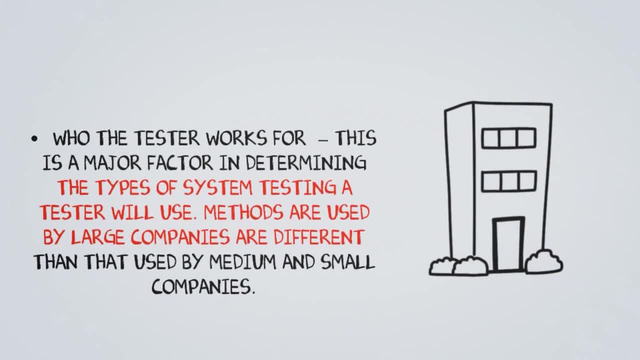 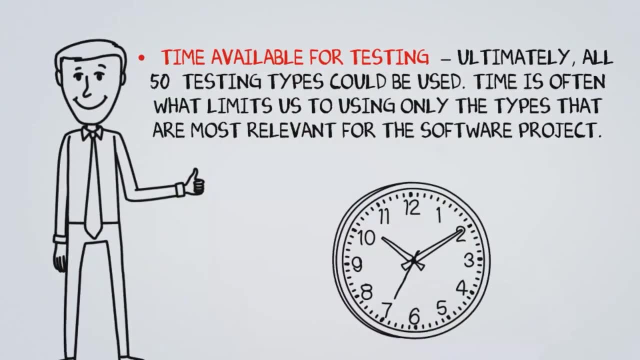 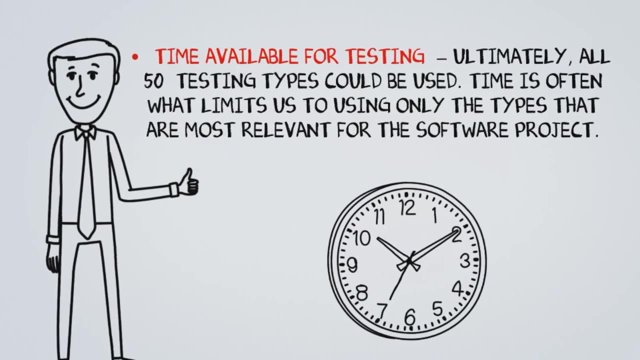 Methods used by large companies are different than those used by medium and small companies. Time available for testing: Ultimately, all 50 testing types could be used. Time is often what limits us to using only the types that are most relevant for the software project. 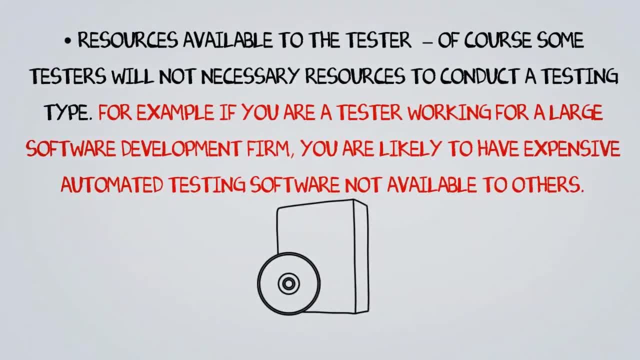 Resources available to the tester. Of course, some testers will not have necessary resources to conduct a testing type. For example, if you are a tester working for a large software development firm, you are likely to have expensive automated testing software not available to others. 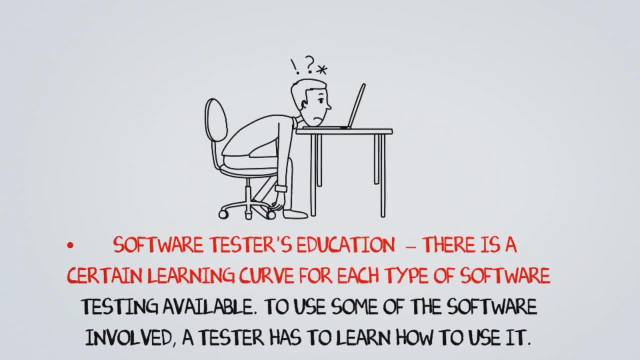 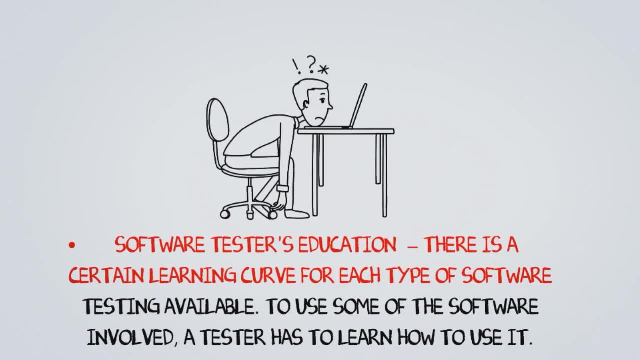 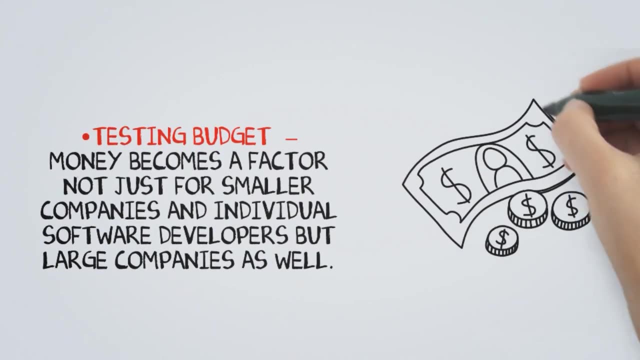 Software tester's education. There is a certain learning curve for each type of software testing available. To use some of the software involved, a tester has to learn how to use it, And testing budget Money becomes a factor not just for smaller companies and individual software developers, but large companies as well. That's all to system testing.